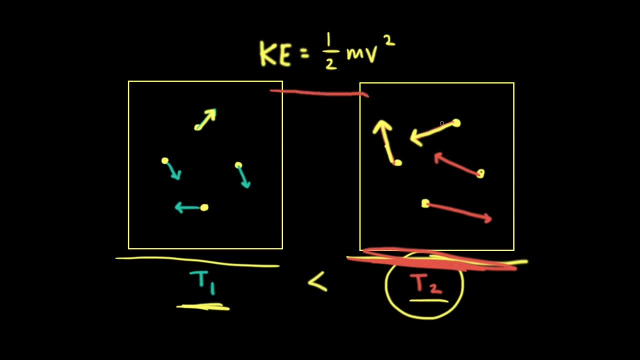 the average kinetic energy of the particles in the box on the right is higher than the average kinetic energy for the particles in the box on the left, And so the average kinetic energy is proportional to the temperature. The higher the temperature, the higher the average kinetic energy of the particles. 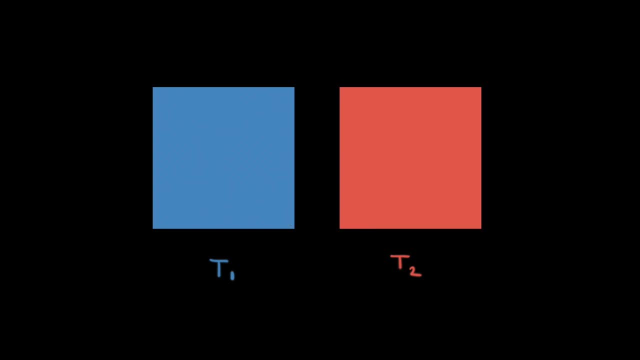 Instead of gases. let's look at two metal blocks made of the same material. So one of the metal blocks is at temperature T1, and the other metal block is at temperature T2.. Let's say the temperature T2 is greater than T1.. 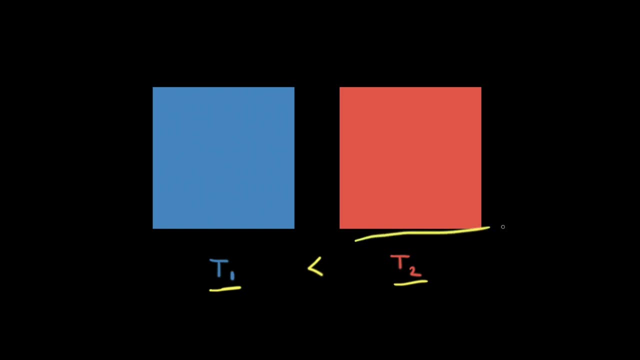 What that means is the particles in the metal box on the right are, on average, moving faster than the particles in the metal box on the left, And that means that the average kinetic energy of the particles in the box on the right is greater than the average kinetic energy. 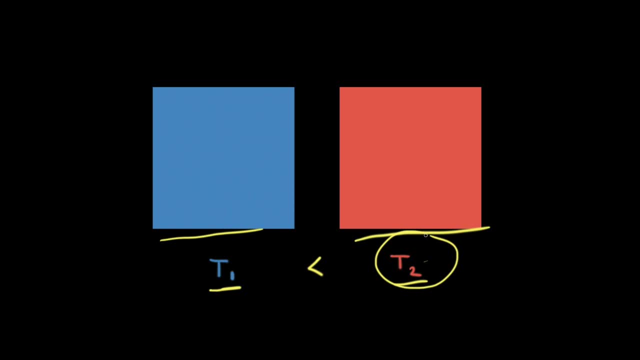 in the particles in the box on the left. Also, notice: right now our two pieces of metal are not touching each other, So there's a little bit of space between them. Next we bring the two objects and we put them in contact with each other. 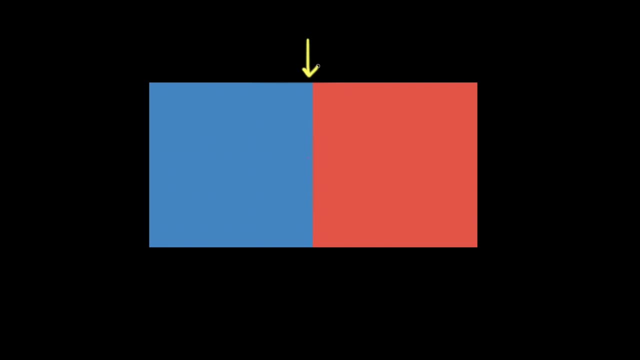 So now there are collisions between the particles that touch And this results in the transfer of energy from the hotter object to the cooler object. So heat flows from the object at the higher temperature to the object at the lower temperature, And so the hot atoms in the metal object on the right 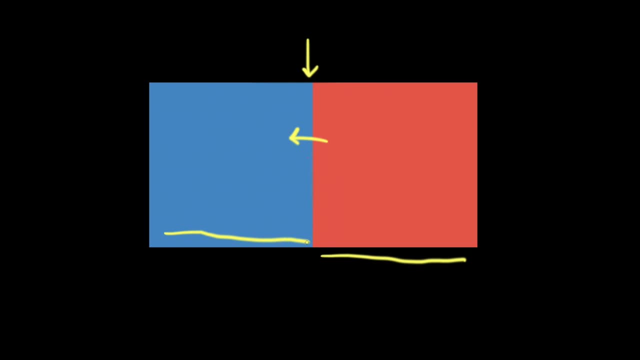 start to move slower, whereas the colder atoms in the metal on the left start to move a little bit faster And the transfer of energy continues until both objects have the same final temperature And we say that thermal equilibrium has been reached. So here we have our two objects. 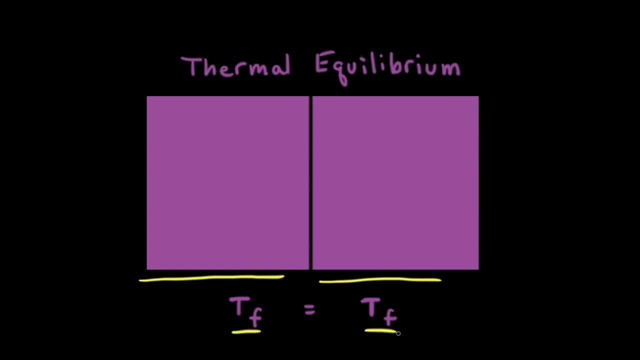 and the two objects are at the same final temperature, which means we have reached thermal equilibrium. And since we've reached thermal equilibrium, there's no more flow of heat between the two objects. And since both objects are at the same final temperature, that means the average kinetic energy of the particles. in both objects is now the same.